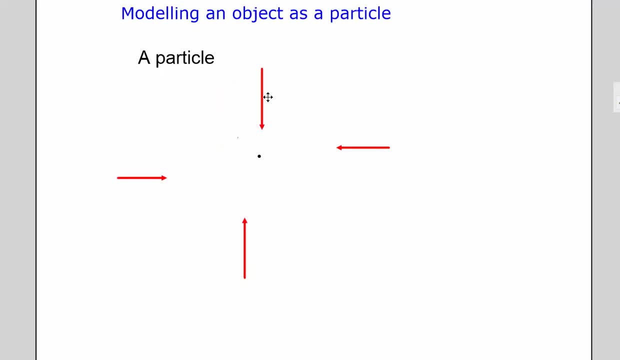 And we've got some forces acting on that particle. So let's say we've got a force pushing it down And then we've got another force, an equal force, let's say pushing it up. I'll just move those And they're equal forces. let's say so now it's not moving. 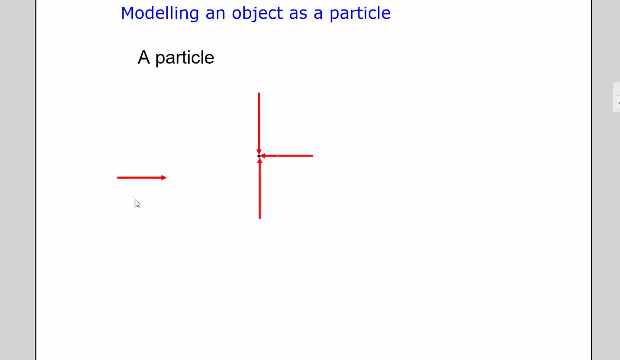 And then let's say, we've got another force pushing it to the left, and then another equal force pushing it to the right, And now we can see, because it's a particle, all of those four forces are acting at that single point. 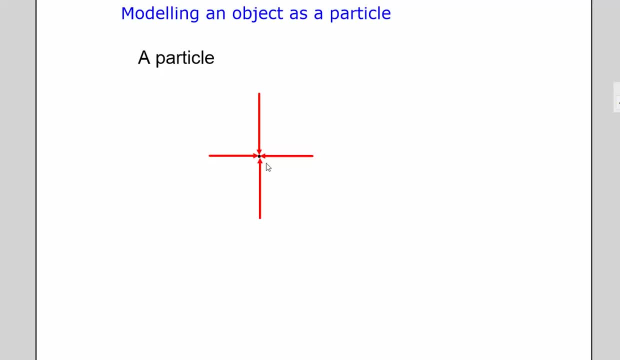 And that's very useful when we're creating a mathematical model and trying to form equations. So one of the, or the main thing related to modelling an object as a particle is the fact that all the forces are acting at a point. Now. if we have a larger object that we can't realistically model, 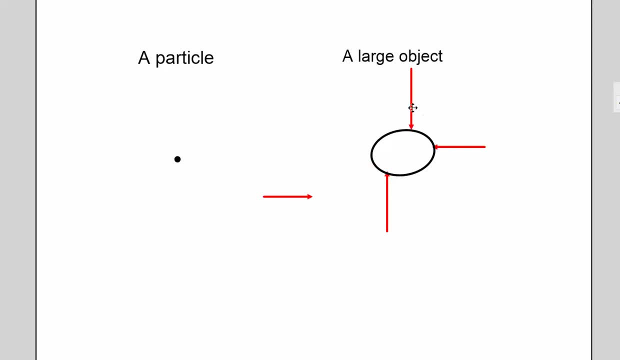 as a particle. what happens? Well, we've got our four forces that were all acting at a single point when it was a, when it was a particle. But those four forces, when they're acting on a large object, they may not be acting at the same point. 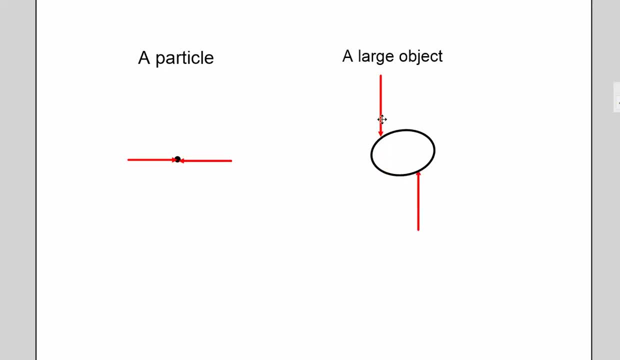 So the upward force might be acting here, the downward force might be acting here, possibly. And if that's the case, what's going to happen to this sort of egg-shaped object? Well, because that one's pushing it down here, this one's pushing it up here. 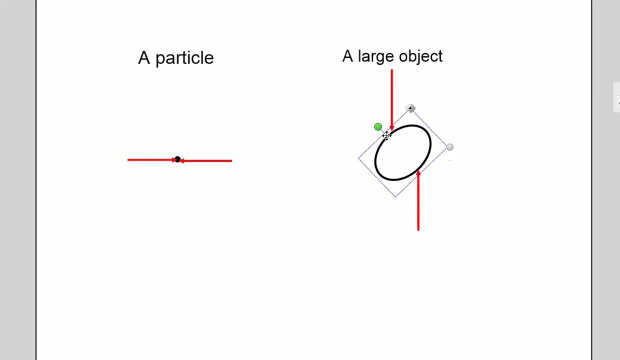 it's probably going to spin round. And then if we get our sideways forces- let's say we've got one here and one here again- that's probably going to make it spin round. So we've then got to take into account. 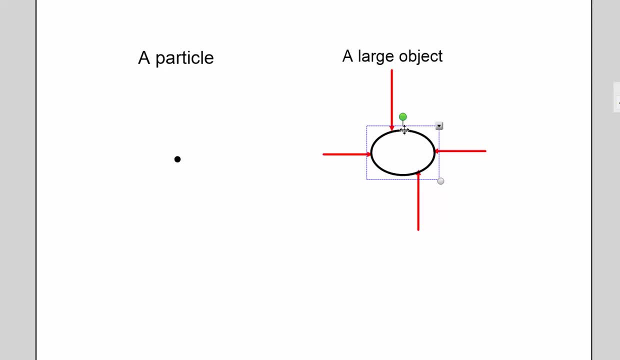 extra things that are happening to that object, and it makes the mathematics a lot more difficult. Now you'll be pleased to know that in the mechanics courses that we do, we're always going to model our object as a particle. Now how would you? 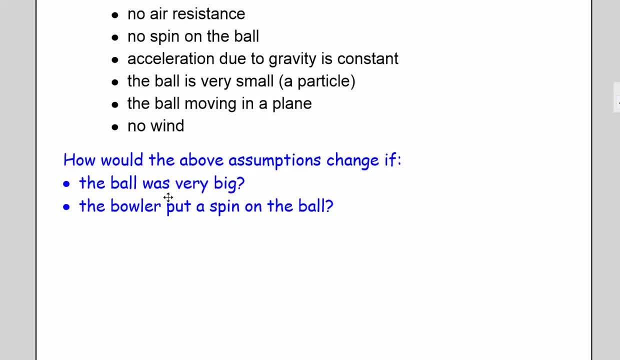 or how would the Bov assumptions change if the ball was very big And if the bowl was very big And if the bowler put a spin on the ball? Now, looking at those, we're probably going to have to change this first. second one here. 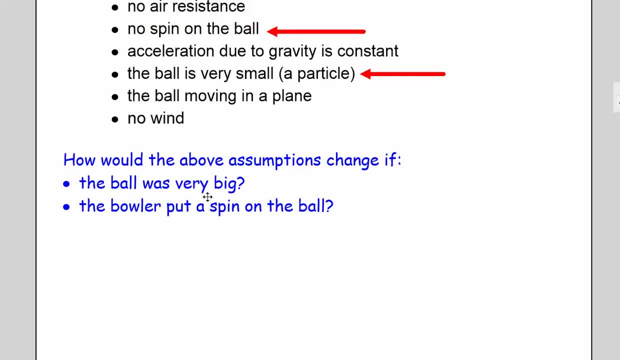 no spin on the ball because obviously we've decided we're going to have spin on the ball, so we've got to eliminate that assumption. We've said it's not a particle, so we're going to have to eliminate that assumption. But we 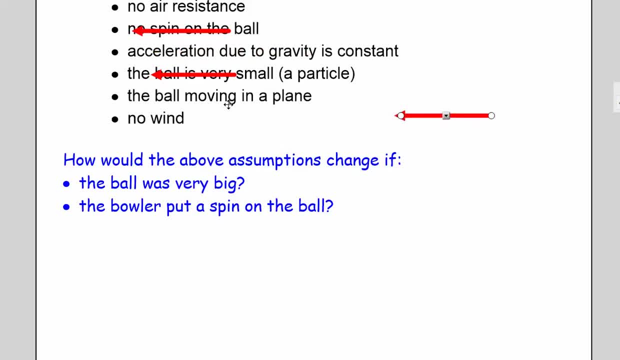 We've also got this one here, that the ball is moving in a plane. Now, if the ball is spinning, it may be moving up and down, but it may be also moving backwards and forwards, so we're probably going to have to. 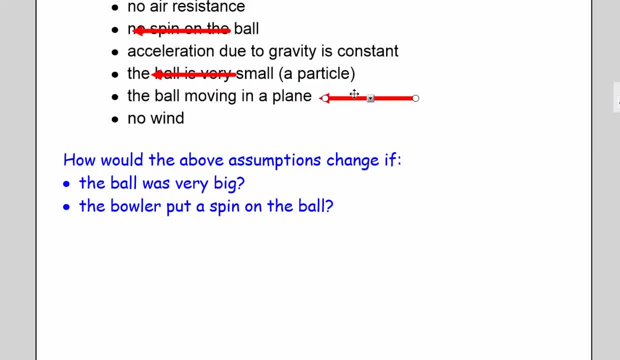 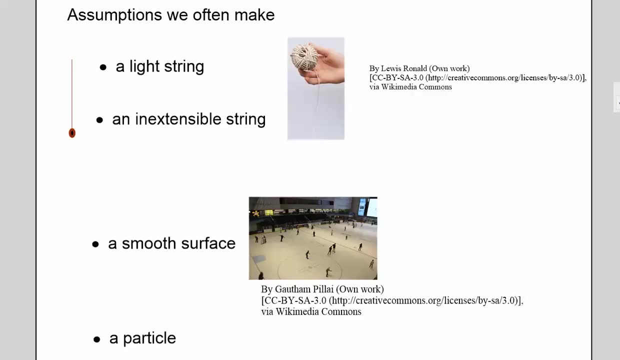 eliminate this one here that it's moving in a plane, because it probably isn't moving in a plane. So the fewer assumptions that we've got, the more complicated the model will be Now, just before we have a look at those, 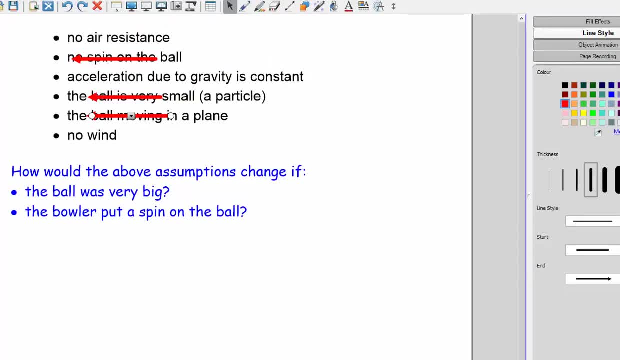 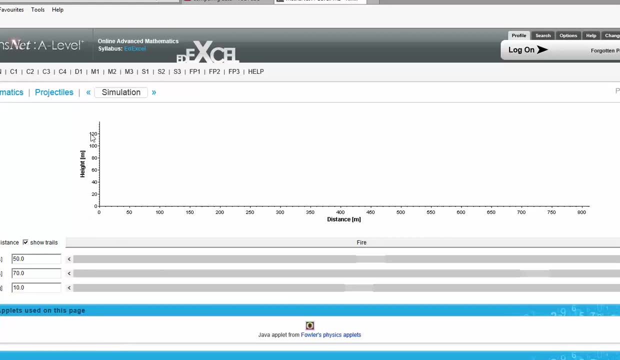 let's have a look at a simulation here. So this is our simulation for throwing a ball, or throwing a ball up in the air. So we can, Because we're working in a single plane, we can use our axes, our horizontal axis and our vertical axis. 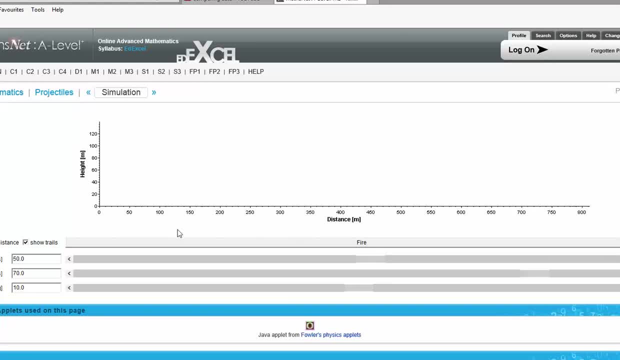 and then we're going to fire the ball. Now we're going to assume as well that it's going to be thrown from this point: 0, 0,. so we're throwing it from the ground and it's going to land horizontally. 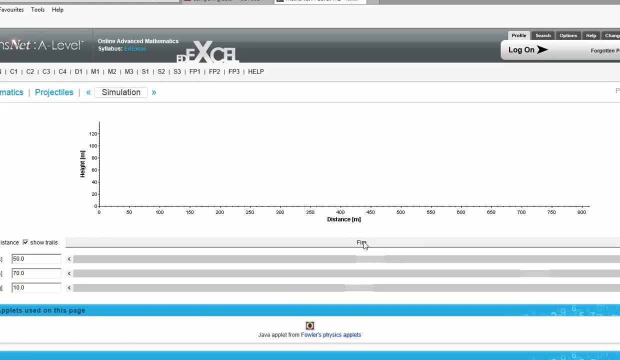 in the same position. So if I fire the ball, here we go And that's our model for a ball, using no air resistance, no spin modelling as a particle And we can probably see actually it forms a parabola.